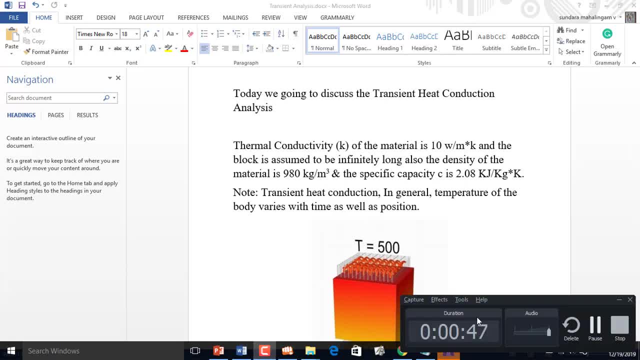 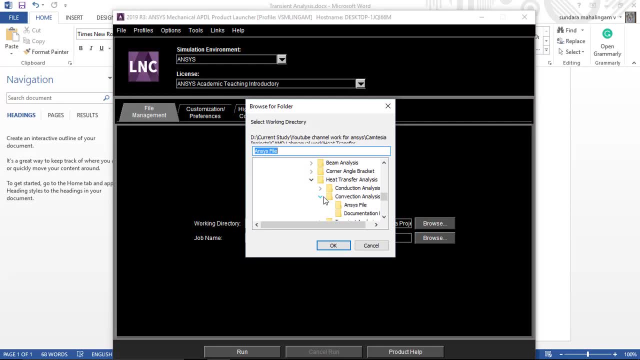 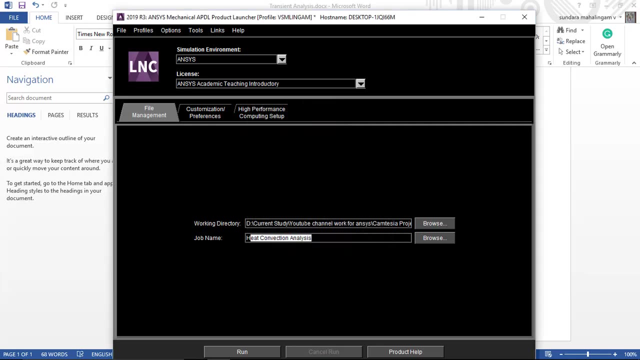 of the block is 10 Watt per m kelvin. As usual, we need to define the directory where all the files need to be stored. Go to there where all the files need to be stored: Transcend heat conduction analysis, ANTSYS file, iqok and transient heat conduction analysis Change. 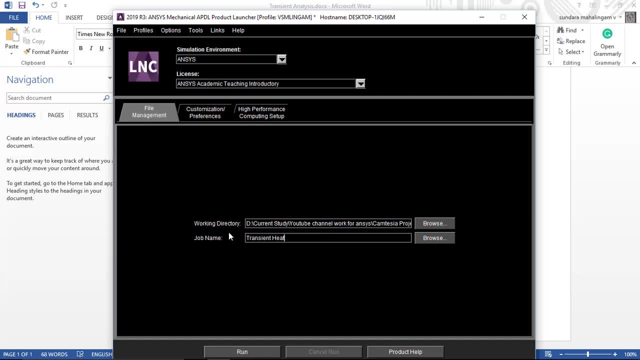 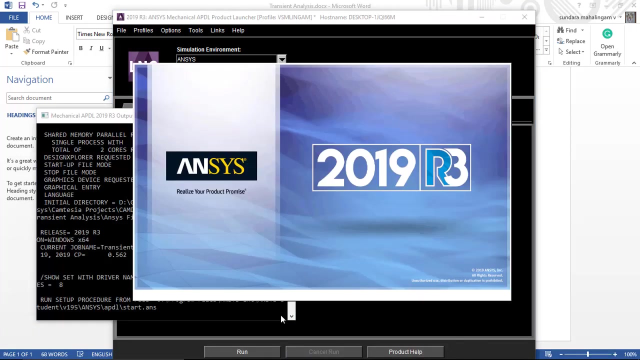 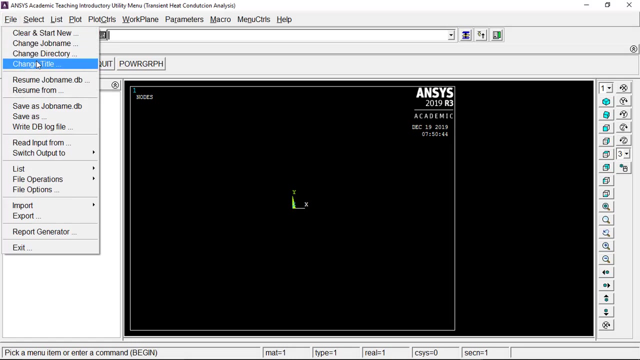 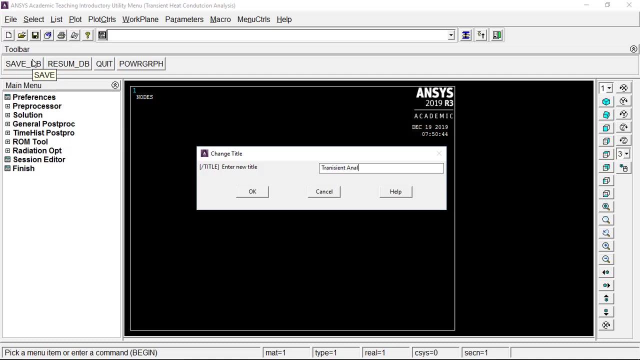 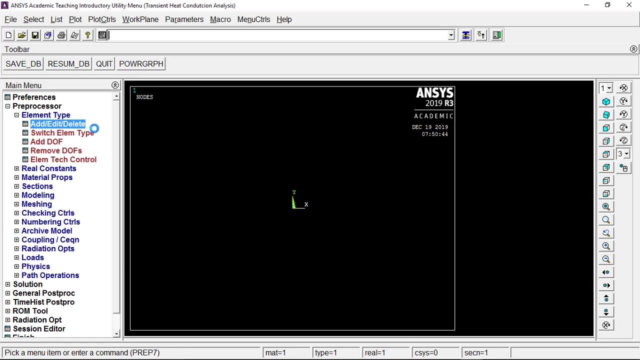 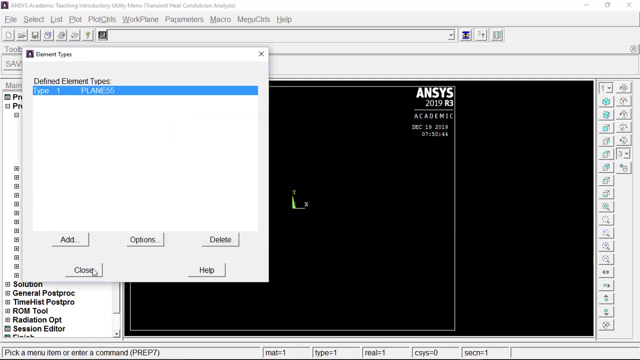 the job name. Just click run. Then change the title: Transient heat conduction analysis. Then give preference, Then choose thermal, Then next go to preprocessor element type: delete. Add Solid Quad 455.. Give ok, Then close. Then go to material property: Material. 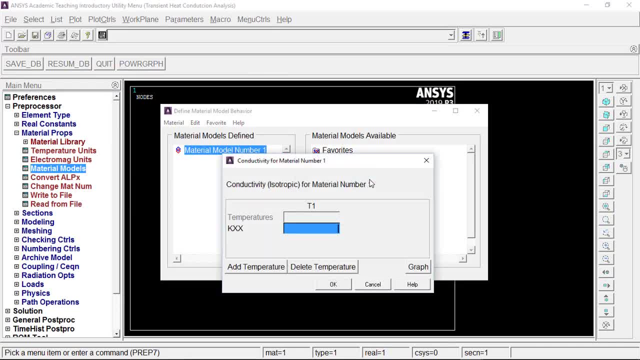 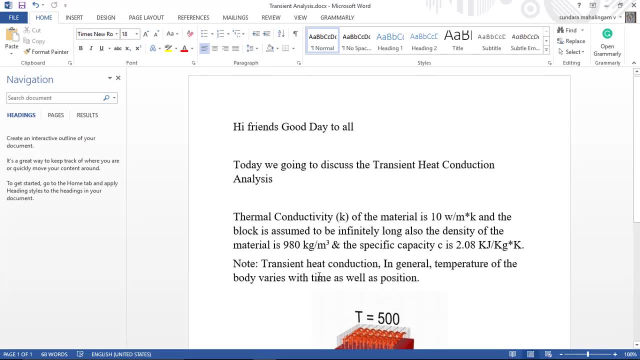 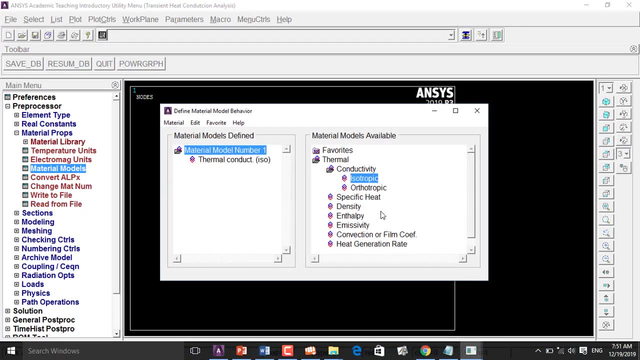 model: Thermal conductivity: isotrophic Thermal conductivity, 10 Watt per m kelvin. So the thermal conductivity given is 10 Watt per m kelvin and then specific capacity: 2.08, and then density of the material: 980 kg per m cube. 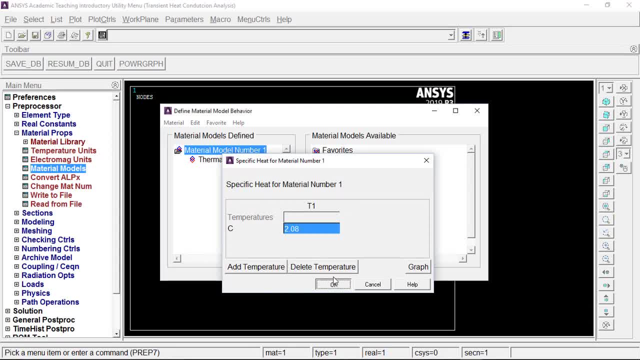 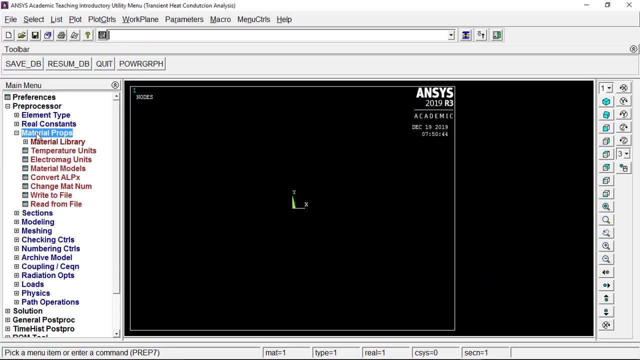 Then give ok, Then close. Next go to modeling. Create Areas: Rectangle By two corner. The center should be 0,0.. The corner should be located 1 meter And then height should be. width should be 1 meter. 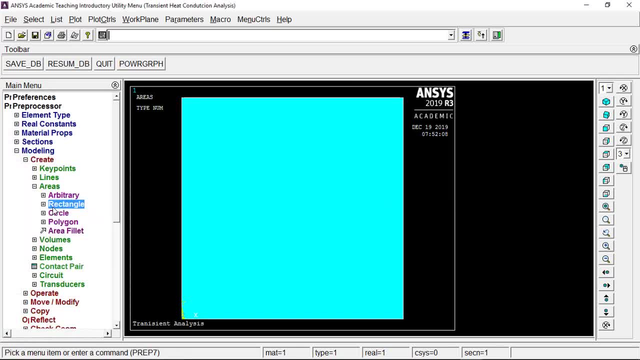 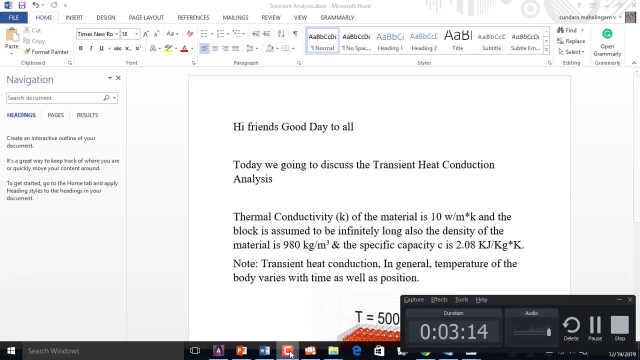 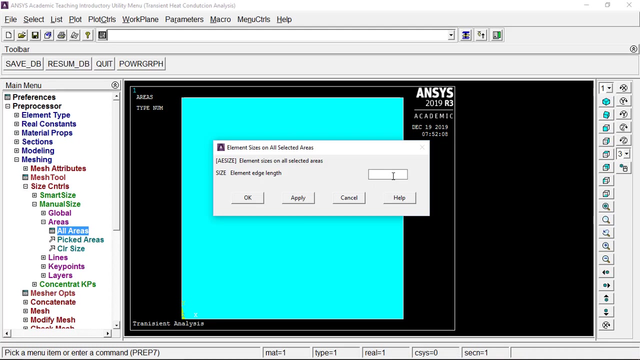 Then give ok. You create the area. Next we going to mesh it. Go to meshing Size control. Smart size- Manual size Area: All area. wait a minute. Smart size- manual size- smart control- manual size areas: all areas. the area should be 0.01.. I just discretize into each and every. 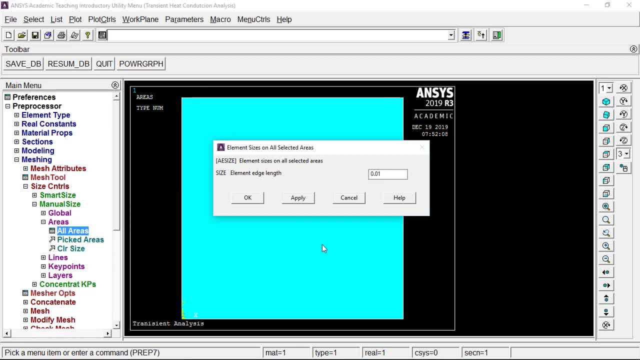 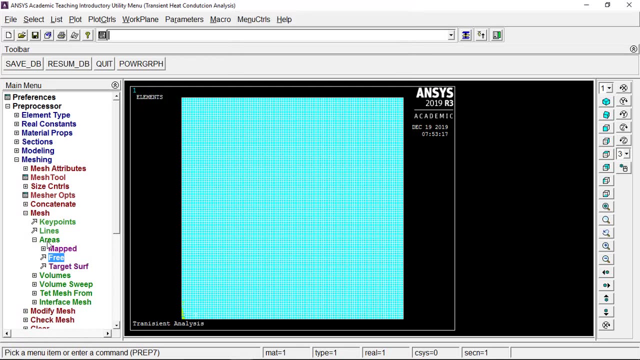 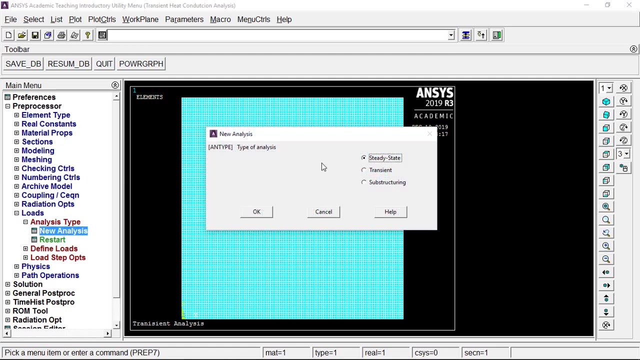 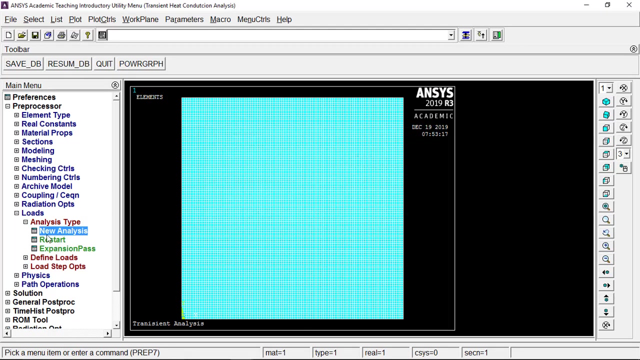 element length is 0.01 meter and then give ok and then next go to mesh areas: free mesh pickle and it will be discretize the element. next go to loads analysis type: new analysis. this should be transient. give ok and then check the solution method is full and then give ok and then next go to define loads. next go to: 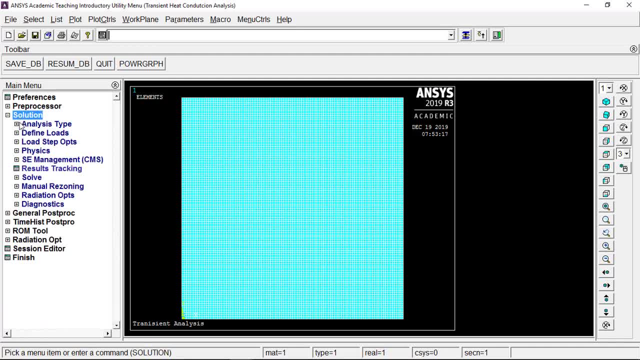 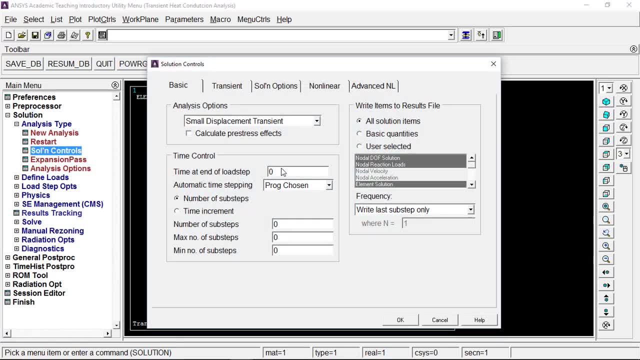 solution. we need to set the analysis type again: analysis type solution control. and then here you need to time at end of load step should be 300 and the number of step steps would be 25 and the maximum number of steps should be 200, and then minimum number of steps should be 25 and then change the. 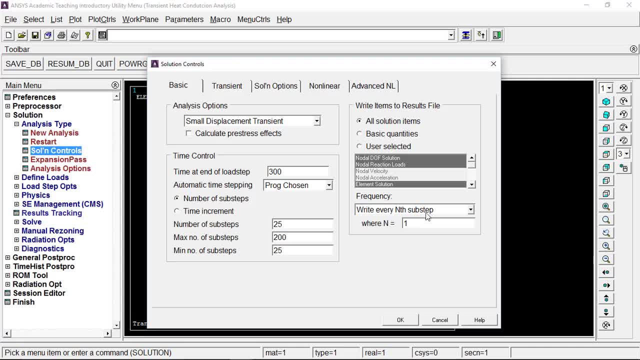 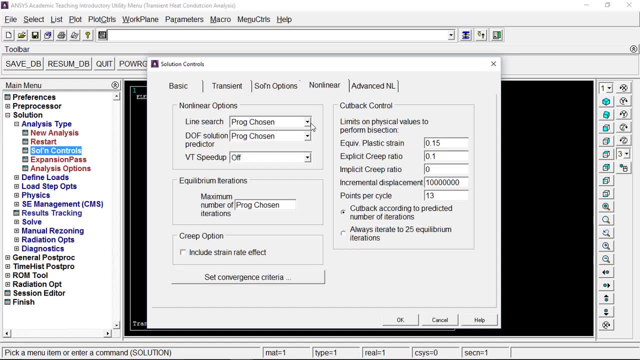 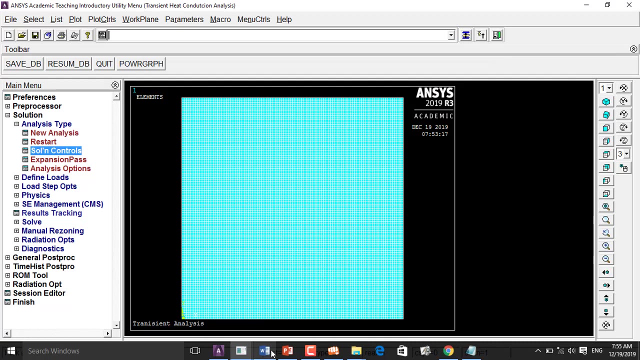 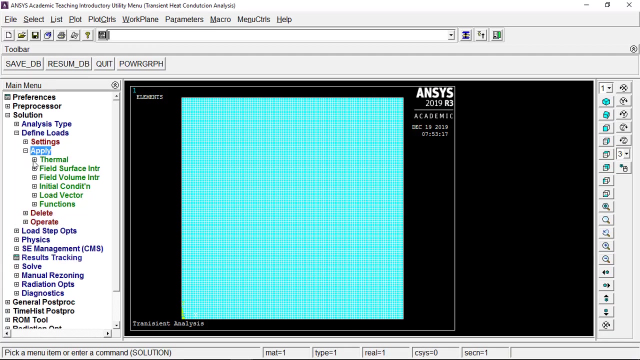 frequency. it should be: write every nth step, each and every nth step. it need to be: calculate the frequency and then go to solution option. go to nonlinear and then enable the line search on and then choose the number of iteration as 100 and then Q. ok, next go to define nodes. apply thermal temperature on nodes. 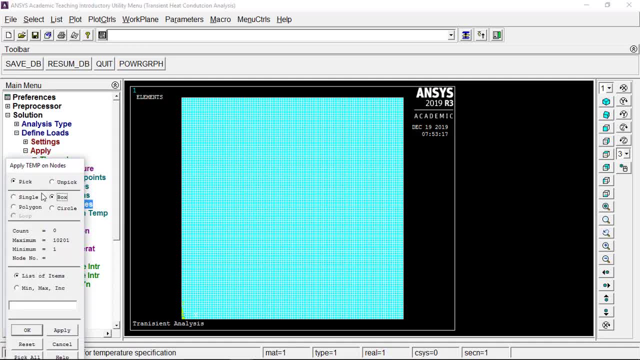 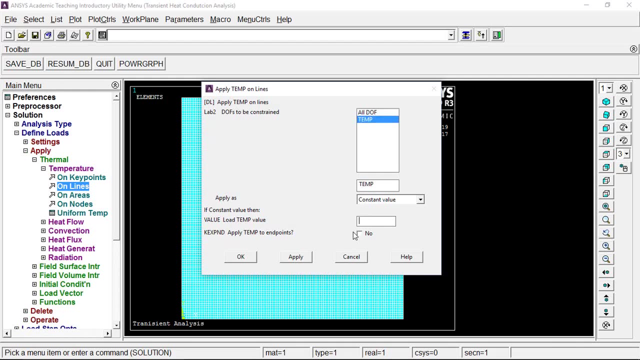 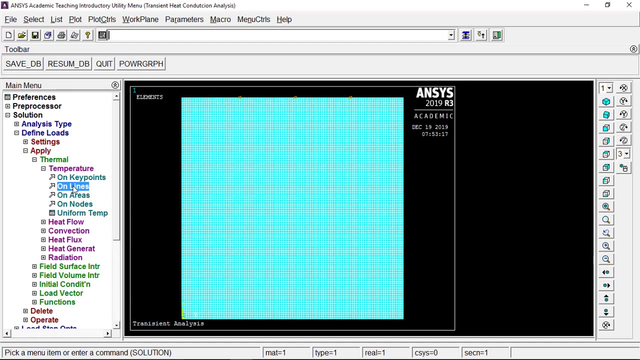 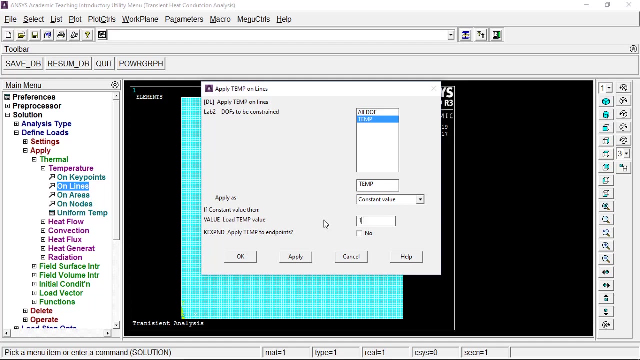 select the box by, or else you can use online. select the top line: Q- ok. temperature will be at top surface is 500 degree celsius Q- ok, and then next. choose online. temperature at the bottom surface will be 100 degree celsius Q- ok, and then next. 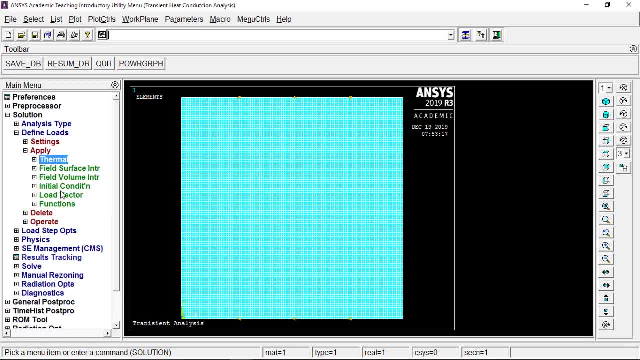 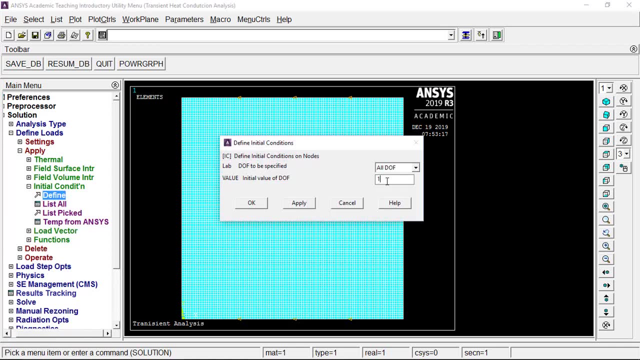 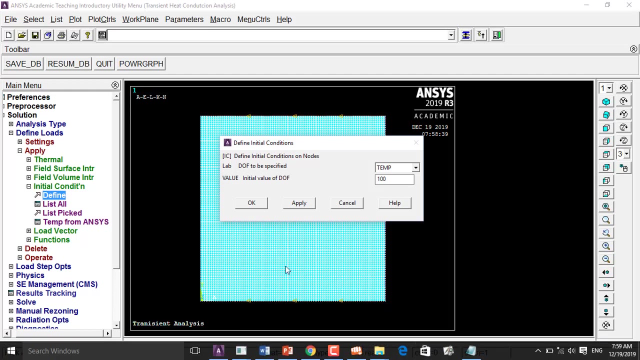 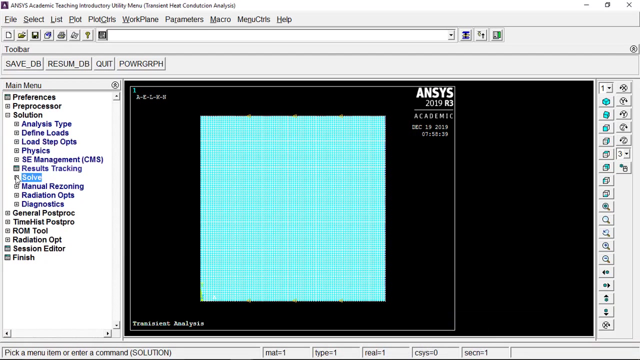 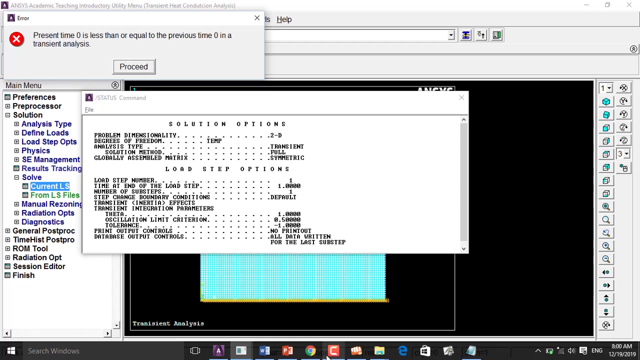 and then choose initial condition. sure, define, pick all, give the temperature value of 100 and then Q: Ok. here you need to change the degrees of random initial conditional temperature, not dof if, and then Q temperature and Press Q ok and then give 100, give ok. next go to solve current tellers. give ok here at. 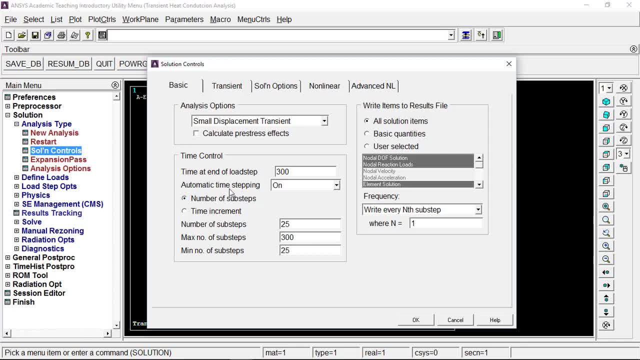 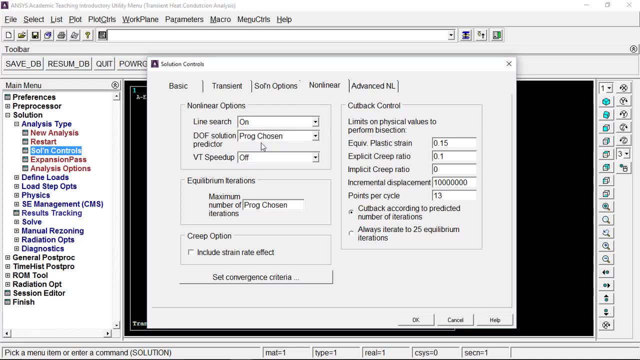 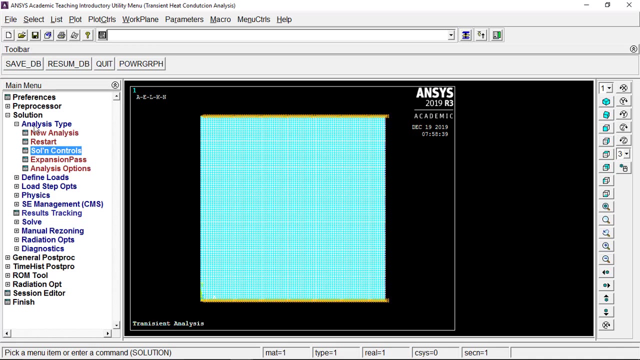 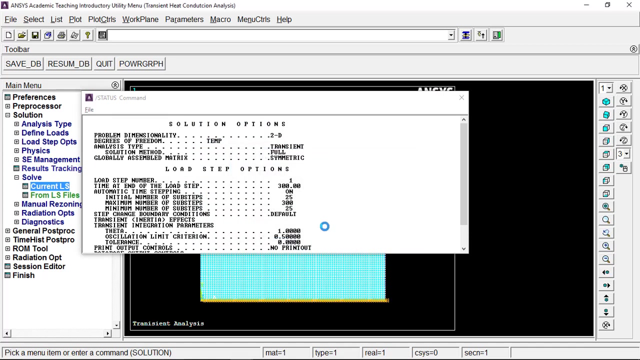 collision control you need to enable. the automatic time stepping should be on, then go to nonlinear and then choose line search should be on and then maximum number of iterations should be 100. no, sorry, number of iterations should be 100 and then give ok and then next go to solution: solve: current tellers. give ok. 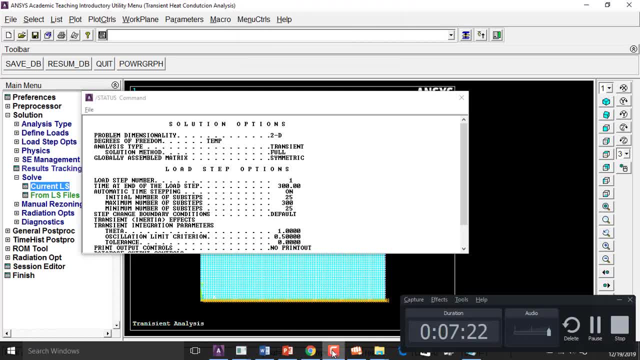 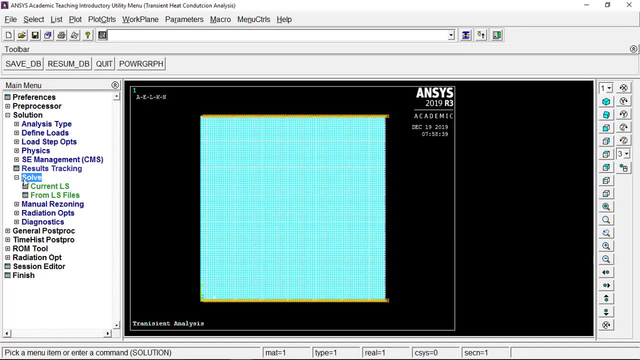 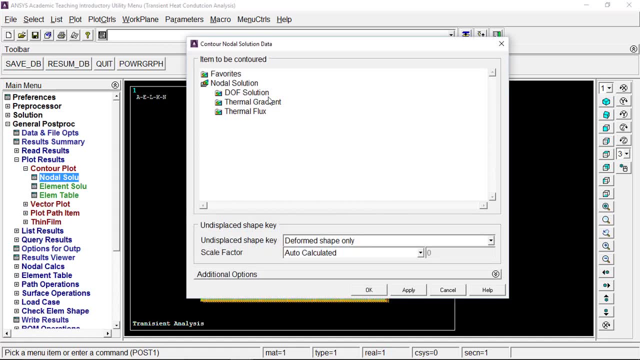 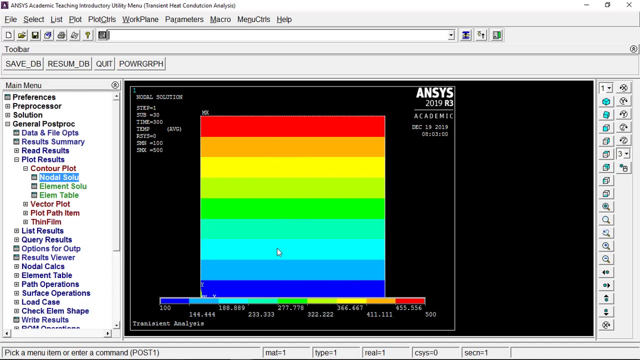 the solution is done. give close. next go to general post processor plot trusses, contour plot, nodal solution. deals of freedom solution. nodal temperature Q K. you can see the temperature variation on this slab surface for the hundred 500 degrees voltage on the top, how the temperature will be. this transfer over the entire surface. go to. 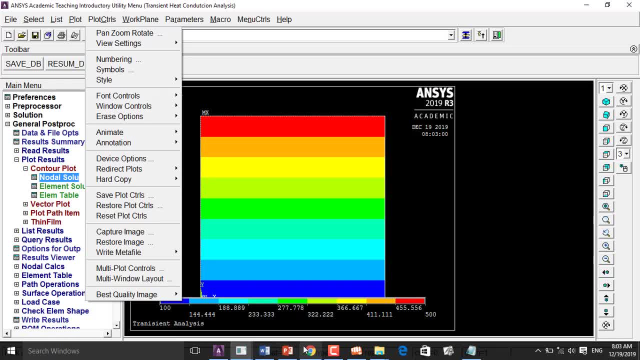 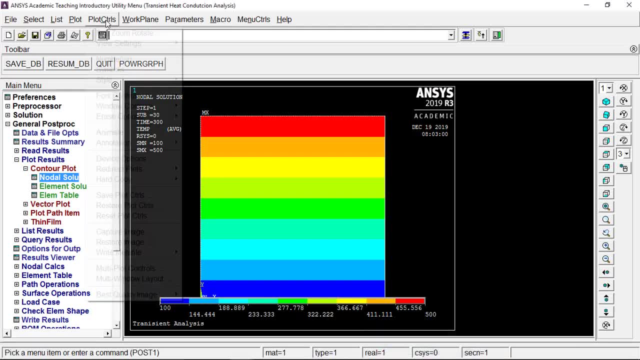 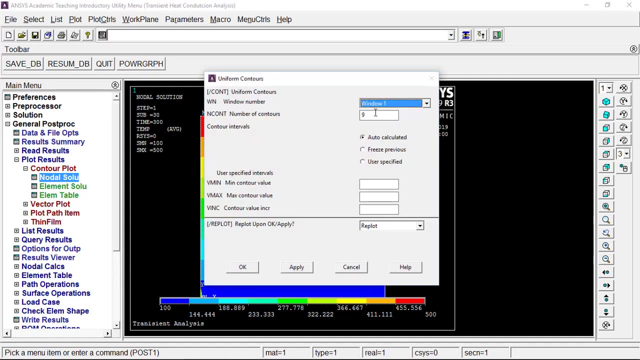 plot control. if you want to see animation or if you want to see the animation over the time, go to plot control. go to plot control, stay. gone to uniform contour Q, the number of contrast line, and then user specified and then minimum number of contour will be 100 uses. maximum contour will be find Danielle, since then. 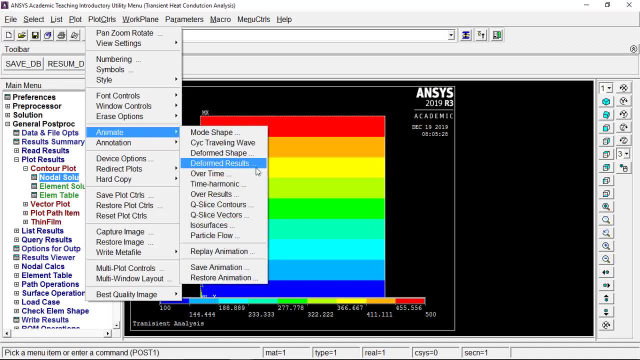 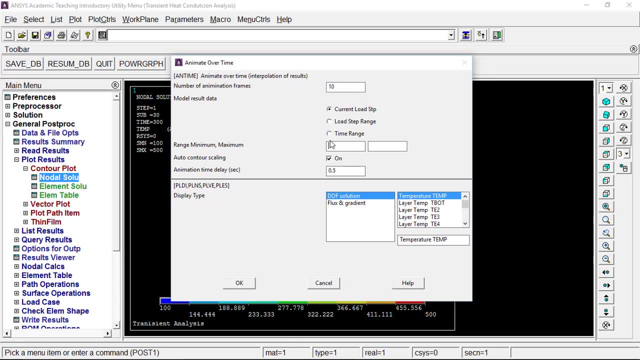 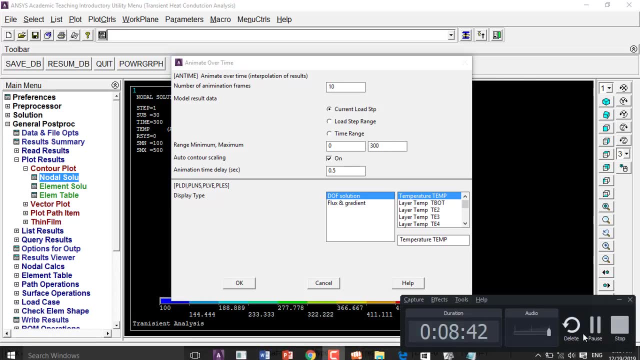 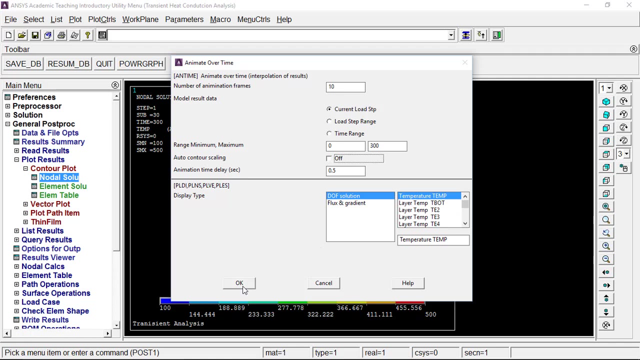 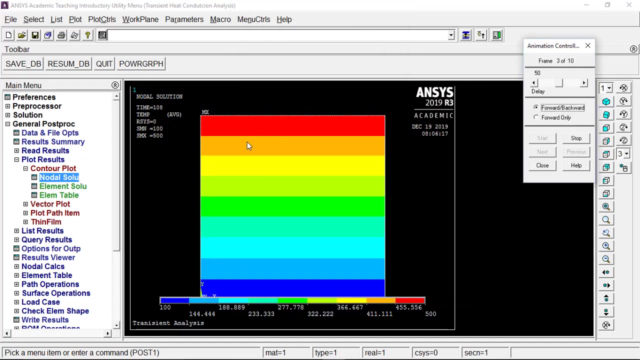 you. okay, go to plot control on имеет over time and then it should be 10. number of animation frames would be 10, range minimum should be 0 and then maximum would be 300. that waist looks contra scaling. D ISA prism solution: temperature give: okay, you can get the simulation of temperature variation on. 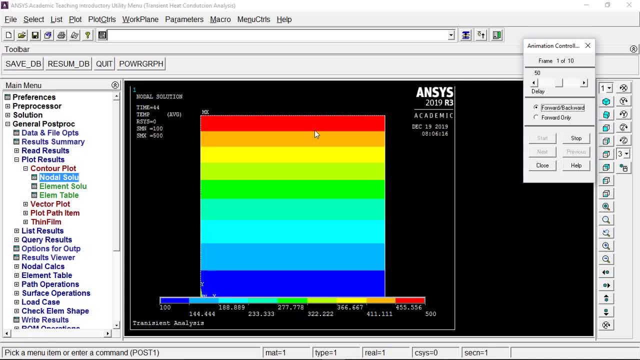 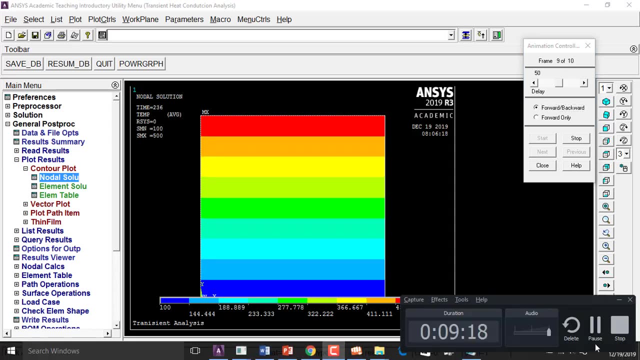 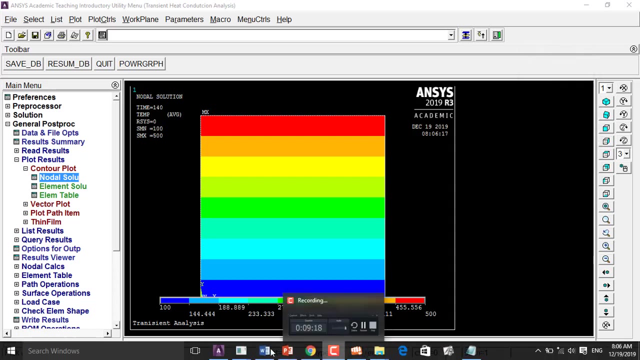 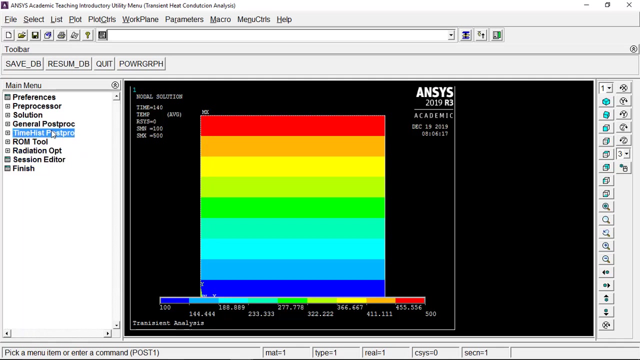 the thermal slab over that time. each and every time frame it shows the temperature vary. now how the temperature will be vary from initial condition 0 seconds to 300 seconds. so it is calculated from 0 to 300. next you can plot the result on the graph. go to time history processor. click the plus mark on. 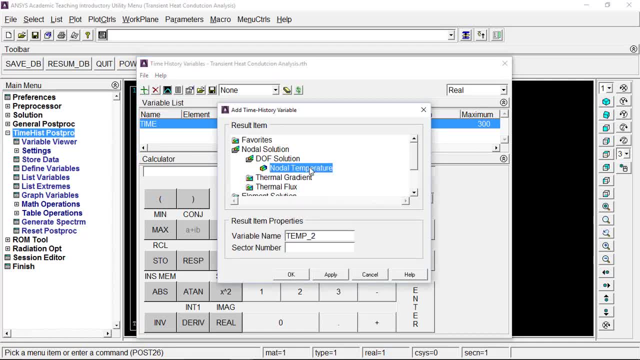 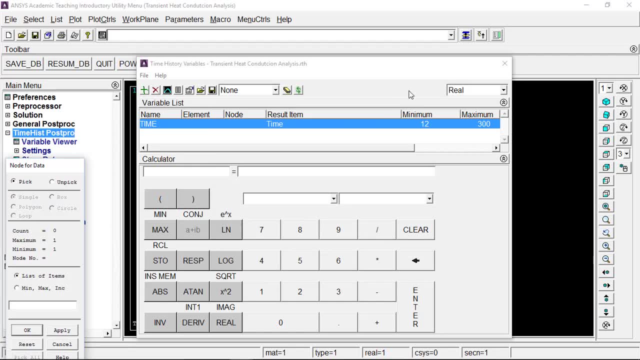 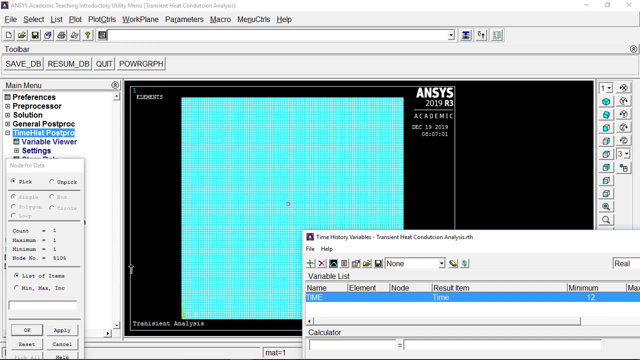 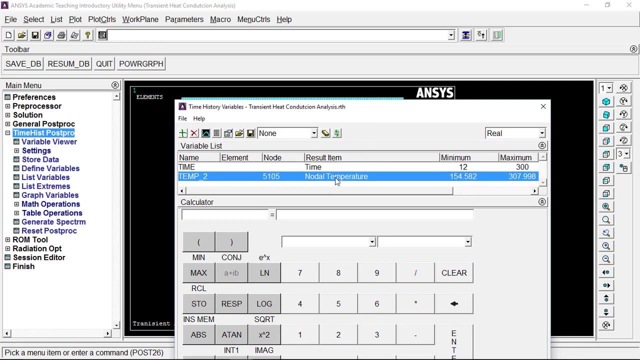 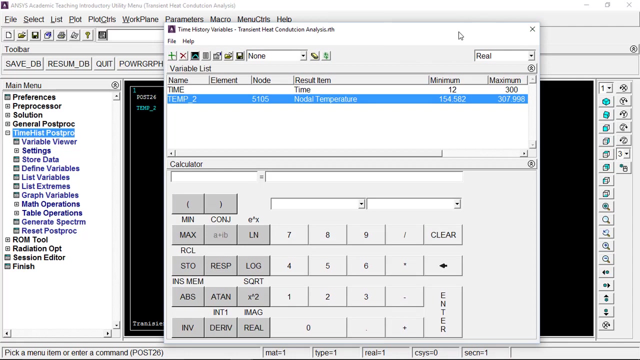 the left top corner: nodal solution- degrees of freedom solution. nodal temperature variable. name should be temperature 2 and then give okay. pick any one node on the mid position and then give okay, ensure the temperature tool to be on. choose the graph. now you can get the graph addresses. here the graph. 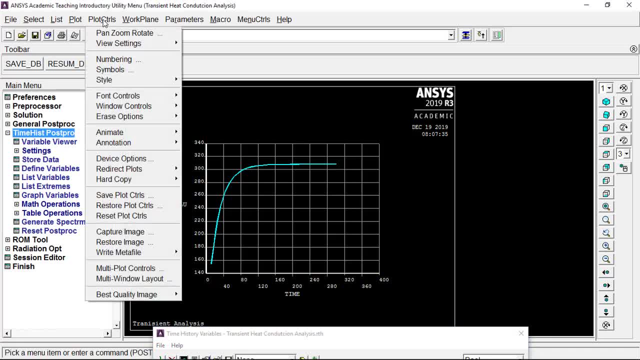 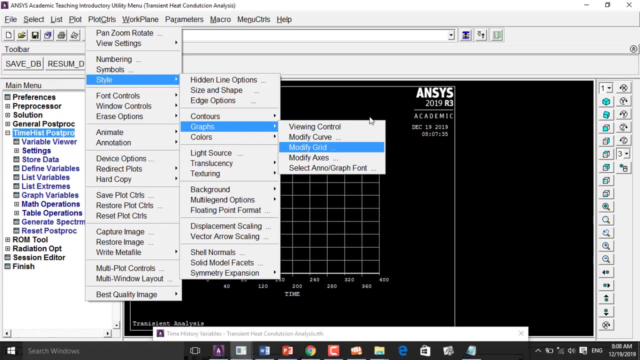 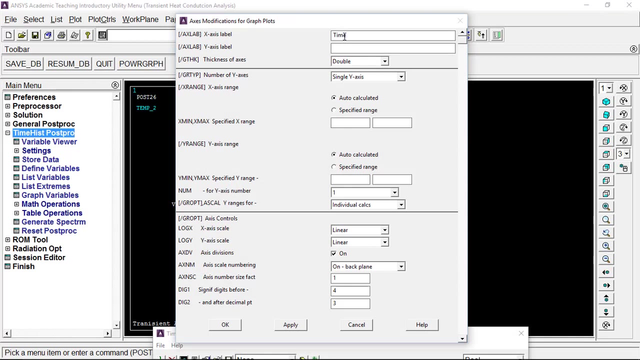 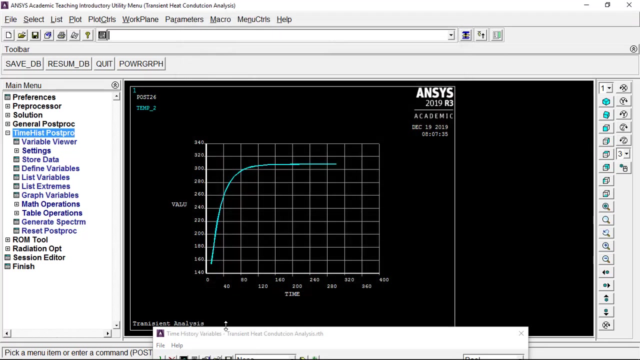 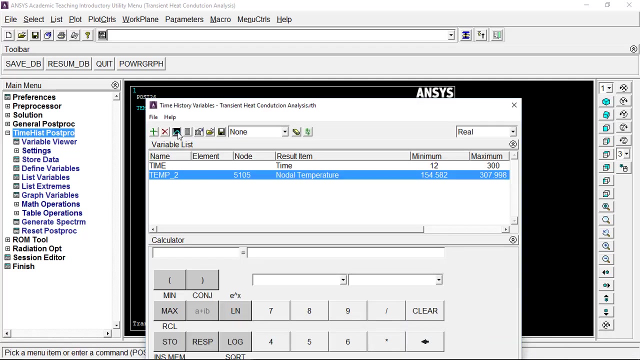 does not change. go to plot control. wait a minute. plot control: style graph: modify curve, modify axis. choose the x-axis label name as time underscore T and then y axis label a surface temperature and then give okay again. choose the graph. here you can see it. label of y axis will be: